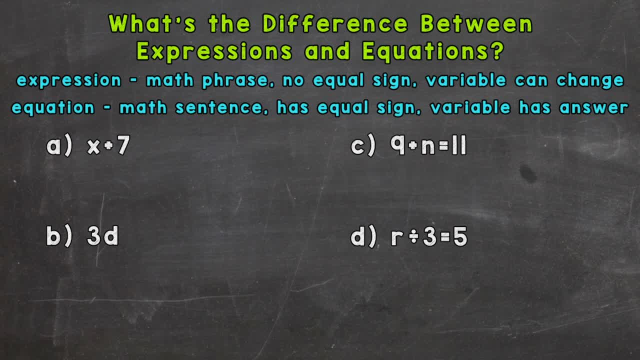 part, And there is no equal sign and the variable can change values. Now, on the other hand, equations are the full math sentence. They have an equal sign and the variable has a defined or set answer. So let's look at some examples in order to make sense of that. So, for examples A and B, 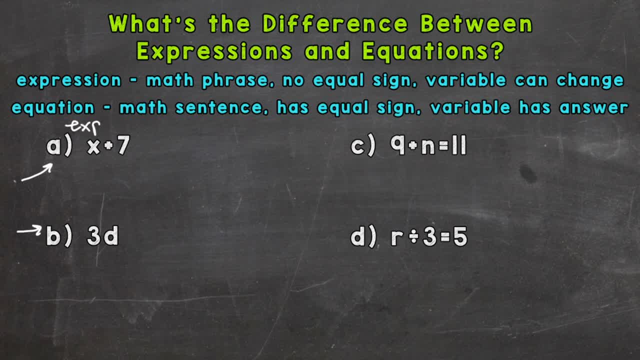 we have expressions over here, So I'll write expressions up here. So, as you can notice, with those examples we don't have an equal sign. They're a math phrase, not the full sentence, and the variable can change. So let's talk about. 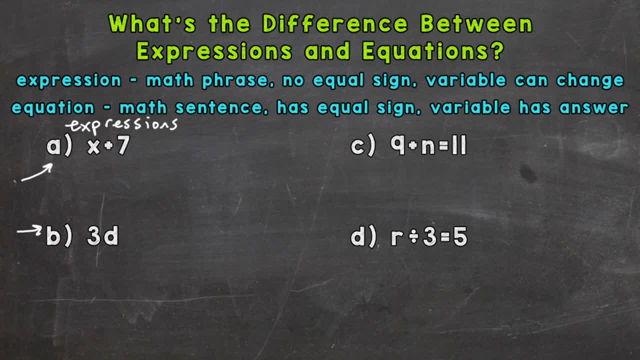 that variable's changing value. So maybe we have x equals 5.. So we have a situation where x equals 5, our variable. So if x equals 5, we would plug 5 in for x and we would get an answer of 12.. 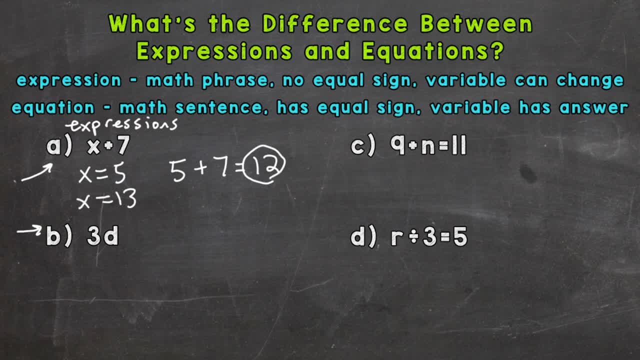 Maybe x equals 13.. So if x equals 13,, plug in and solve. we would get an answer of 20.. So A and B examples of expressions. Now, as far as B goes, whenever you have a letter right next to your number there, 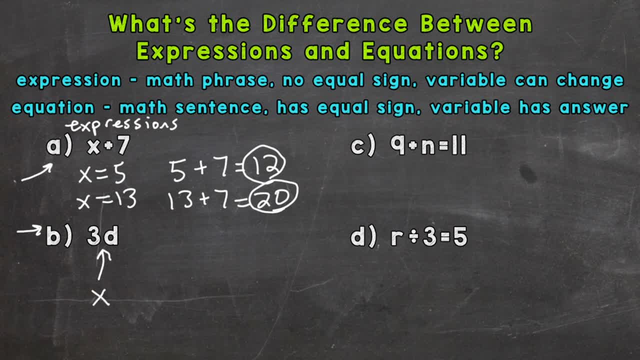 so the number right next to the variable. it's going to be multiplication And let's plug something in. Let's say D equals 20.. So if D equals 20, we would plug in and we would get an answer of 60.. So expressions again, math phrase, not the full sentence, no equal sign and the 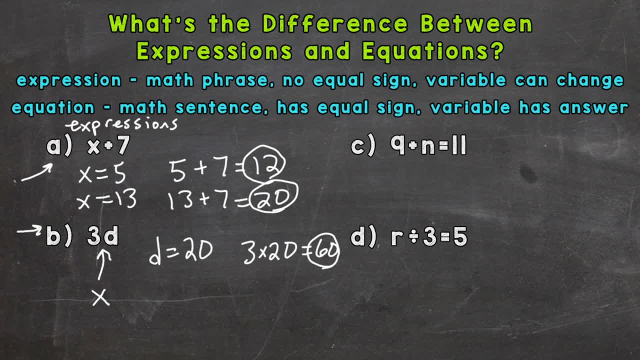 variable can change. So let's move to examples C and D, And both of these are equations. They are the full math sentence, They have an equal sign and the variable has a defined or set answer And a nice, easy way to tell the difference between expressions and equations. equation sounds like equal, right? 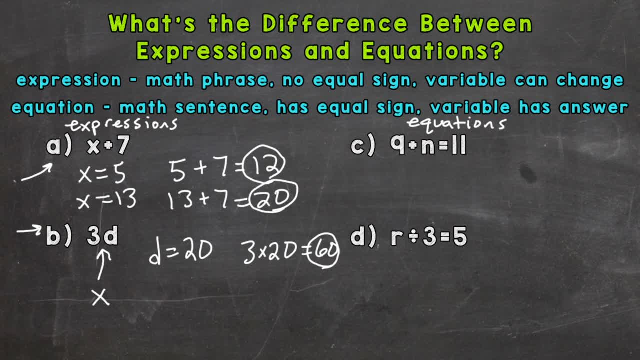 They're similar. So whenever you hear equation you know those are the ones that have an equal sign. So let's talk about the variables. In example C we have 9 plus n equals 11.. The variable's value cannot change. We can't say that n equals 5, because if n equals 5,.